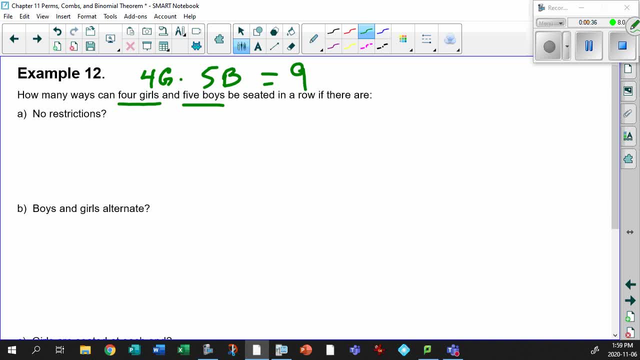 Okay, So a total of nine kids together. Okay, No restrictions. That means you got nine people: One, two, three, four, five, six, seven, eight and nine. Oh, my gotcha Choices for the first one. 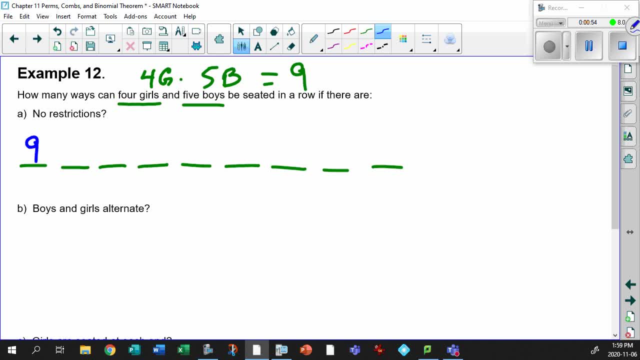 Yeah, there's nine choices for the first one. Choices for the second. There's got to be eight, because there's no restriction. You're just counting down. You got nine kids, Then you got eight kids to seat, Seven kids to seat Six, five, four, three, two and one. 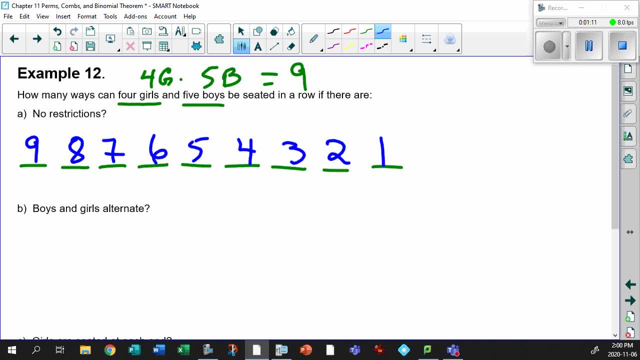 So you're going to just throw this into your calculator and just go Nine times eight times seven times six times five times four times three times one. Oh, my goodness, This actually works out to be 36,000.. No, sorry, 306 seats. 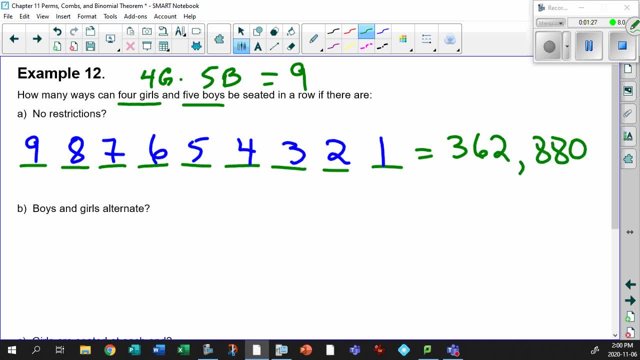 2,880 different arrangements of these kids. I think that's hilarious. I don't think I've ever, as a teacher, went out and went. I have nine kids. I wonder how many different arrangements can I have of these? That's kind of just silly, isn't it? But it's neat to see that it's mathematically. 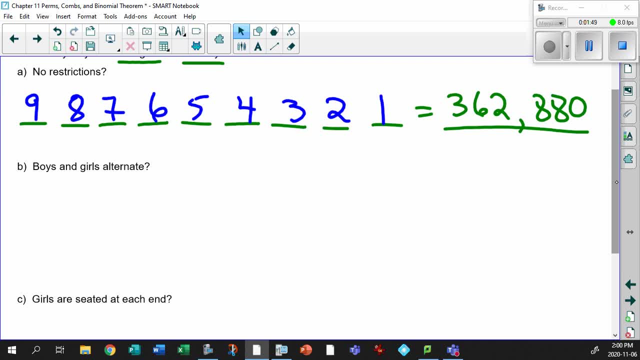 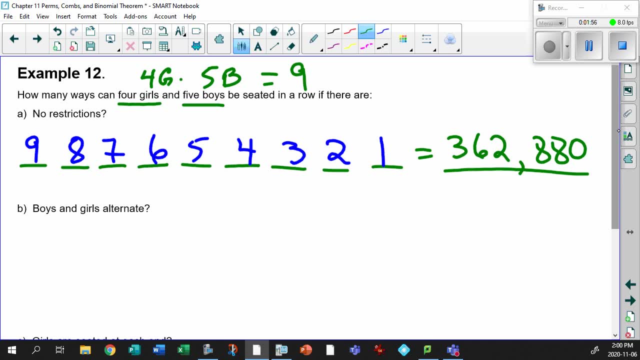 easy to figure out. Now, what happens if boys and girls alternate? Okay, let's go back to this and talk about a restriction here. You got four girls and you got five boys. Now let's talk about this first. If we're going to alternate, think about this- You have to do a little bit of pre-planning. 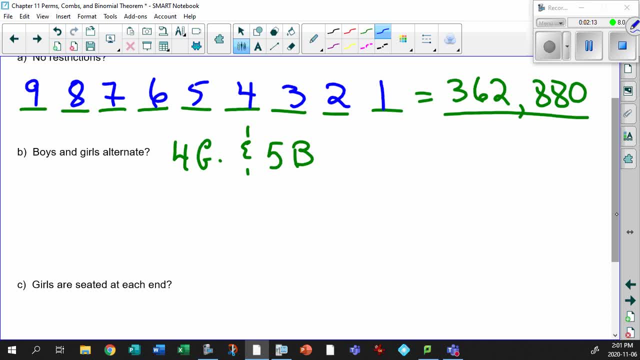 Yes, you still have nine spots, but let's talk about this for a second. Do you start with a girl and then go boy, Or do you start with a boy first and then go girl and alternate? Well, let's talk about this for a second. 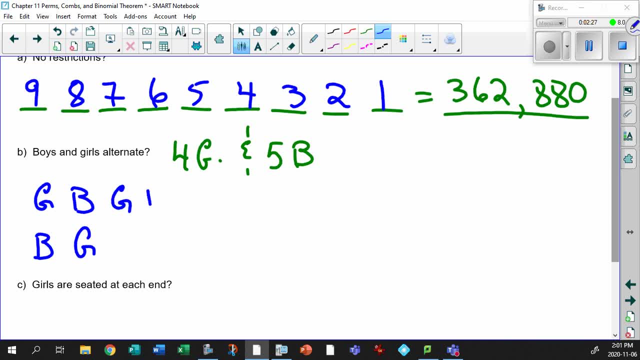 There's girl, boy, Then the next one would be girl, Next one would be boy. So we dealt with three girls so far, two boys, or I should say: two girls, two boys. Okay, There's another girl. There's three girls, three boys. Okay, Four girls, four boys. But okay, so where's the fifth boy? 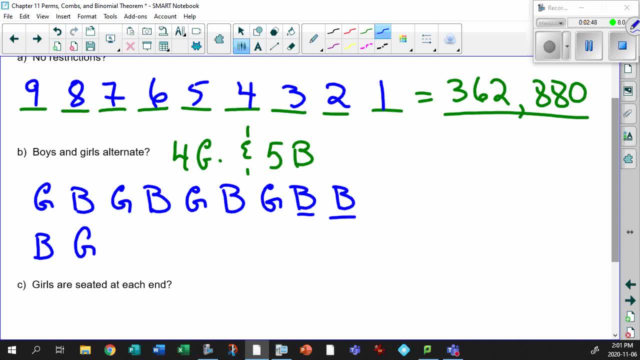 going to be. You can't put them here because they're not alternating. now Think about this: You have to take that boy and you've got to put them all the way at the front. That's the only relationship that you can make that will work, so that they will alternate. 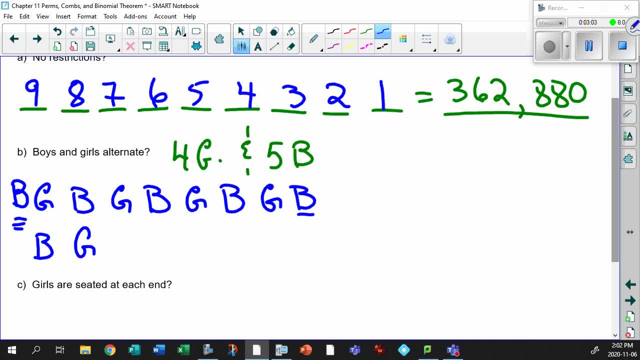 Okay, So you have to start with a boy. So I guess we don't really need to look at this part, do we? Okay, Because we know we got to start with the boys, Okay, So that in mind, let's go, We still. 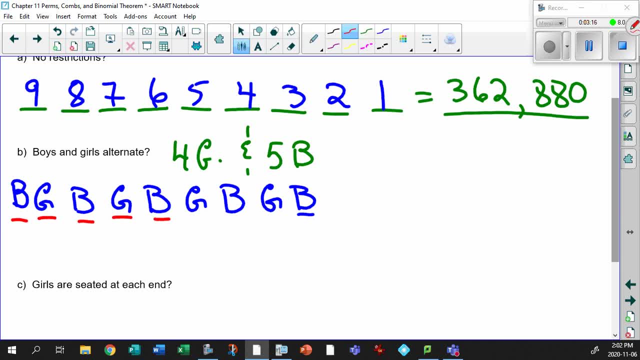 have. look at this: one, two, three, four, five, six, seven, eight, nine positions that we have to deal with. Let's deal with the restriction. The restriction, then, is boys. Boys have to go first. So how many choices do you have for this first boy, Five, Followed by this: 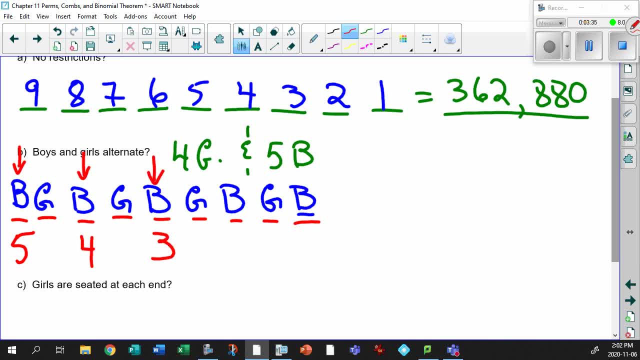 choice Four. Followed by this, choice Three. Followed by this, choice Two. Followed by this choice would be one. Right Now, let's bring in the girls. How many choices for this one here? Well, four choices for here. Three, two, one. Do you see why we have that map? 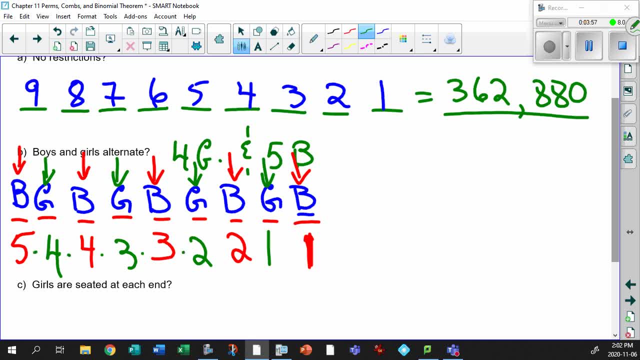 Four, Followed by this choice: Three, two, one. Do you see why we have that map? Five, two, one. Do you see why we have that map? Four, Followed by this choice: Three, two, one. Do you see why we have that map? 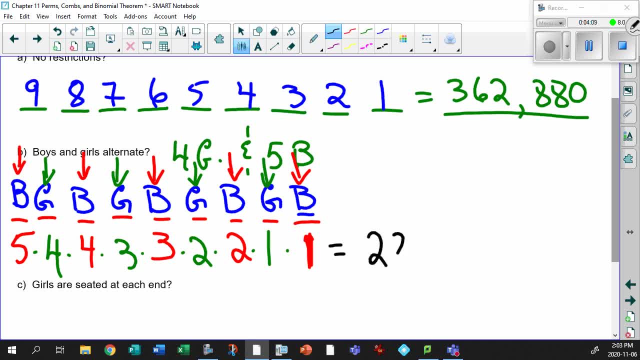 Five, Followed by this choice: Three, two, one. Do you see why we have that map? Okay, So we look at this and that's 2,880.. That's what this number works out to be, And I'm trusting. 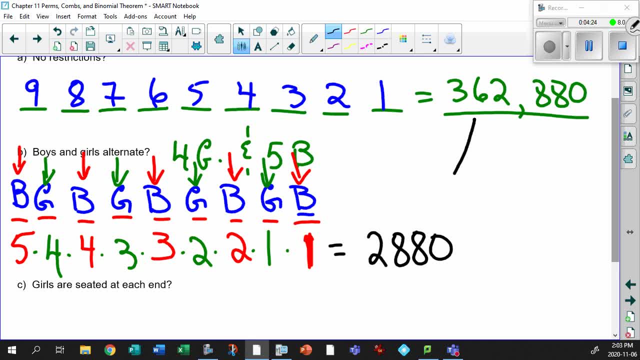 that you're throwing this in your calculator and cranking them out. I'm just not going to bother you. put a restriction on it. look how many fewer arrangements you can make. oh my, that's incredible. okay, so look at my last one. here the girls have to be. 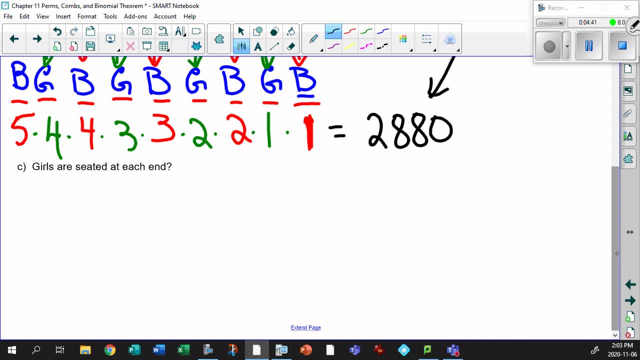 seated at one end. they have to see them all together and they have to be either on the left end here, so this has to be all girls here, right, and this has to be the boys. now listen to this word, or you can put the boys here and the girls. 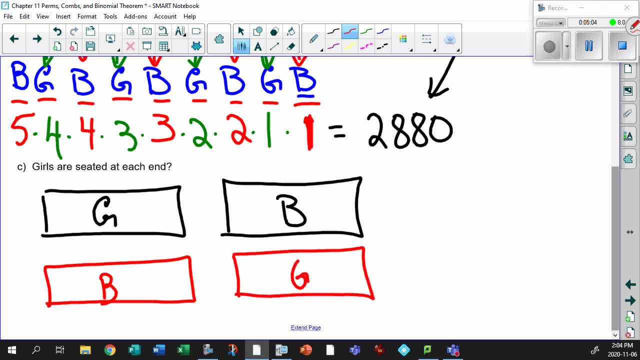 here uh-huh. so we got an or question, so we know we're gonna have to add them. my question is this: okay, girls are seated each end. think about this: how many different arrangements of the girls can you have here? okay, well, you have four girls: one, two, three, four. 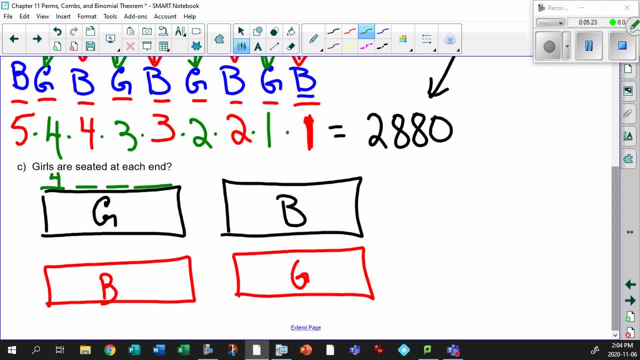 you can have four girl or four choices here. three choices here, two choices. one choice here: okay. and if you multiply that out four times three is twelve. twelve times two, that's twenty four. twenty four times one is twenty four. arrangements here: okay, think of the boys. now the boys can turn around and you can. 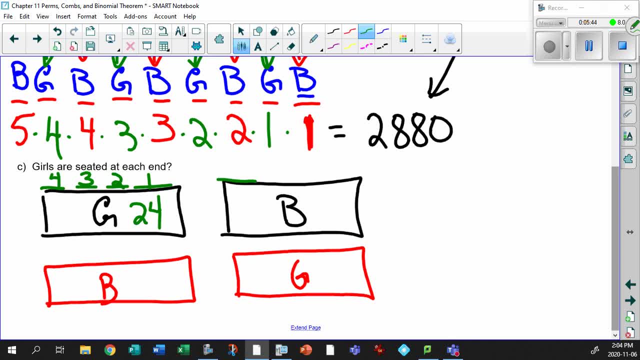 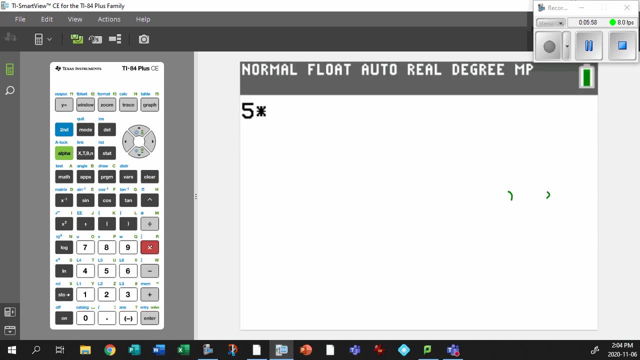 have guess what? yeah, five boys here: one, two, three, four, five. you can have five choices here: four, three, five, 2 and 1.. Multiplying that out: oh, I don't know- 5,, 4,, 3,, 2,, 1.. Let's do it 5 times, 4 times 3. 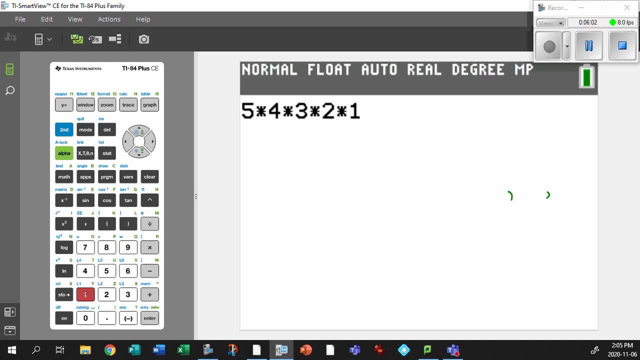 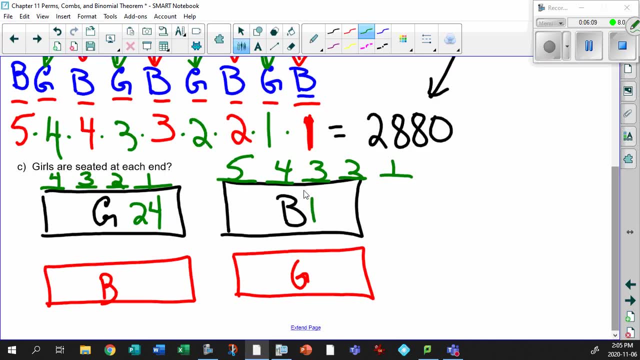 times 2 times 1.. There's got to be an easier way. Oh yeah, I'm going to show you later. Okay, that's 120. arrangements of the boys. right here, There's 120.. Multiply these two numbers together. Guess what You get: 2,880 again. Oh, it's interesting that it's exactly like that. 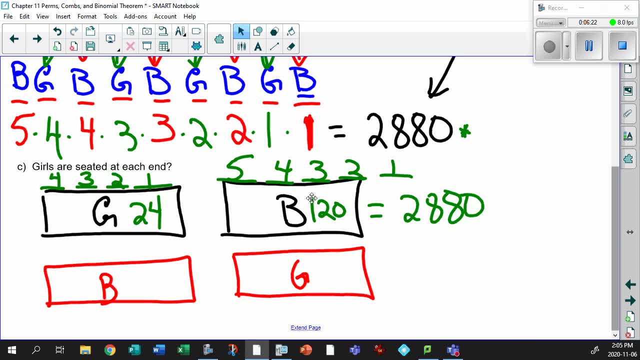 number. But now think about the same thing again. But now we flip them. Girls can be on either end. It could be on the left end or on the right end. Here they are on the right end. Aha, So did the. 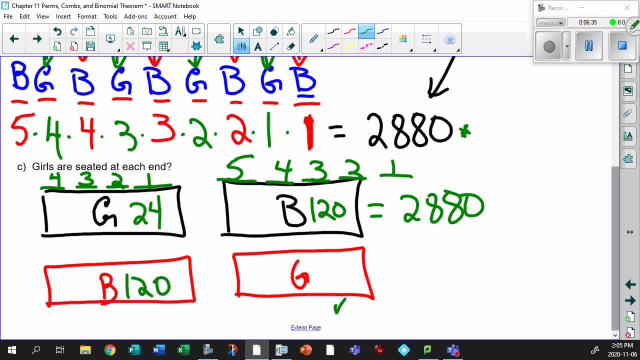 arrangements change. No, there's still 120 arrangements for the boys. There's still 24 arrangements for the girls. Multiply that out, That gives you 2,880 again. But remember you can have the girls on this end or the girls.